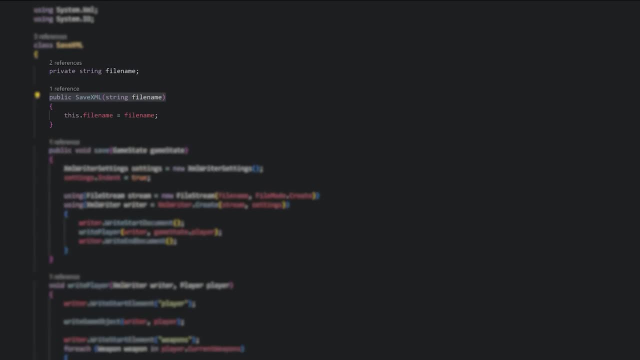 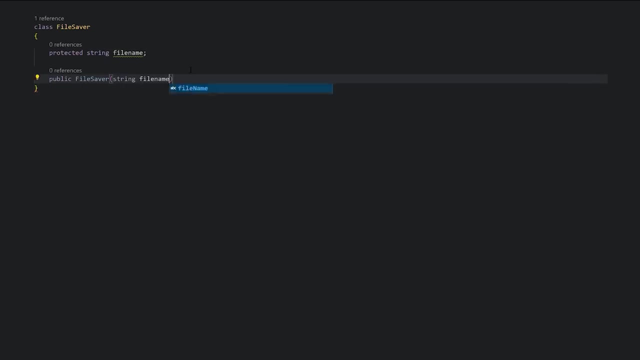 We might notice that both take in a file name. during construction, Our little repetition detectors go off and realize that maybe, maybe we could extract this out. So our instinct is to create a common class called filesaver that just takes a file name. 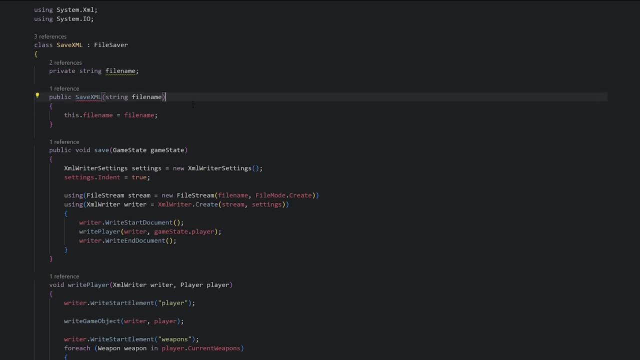 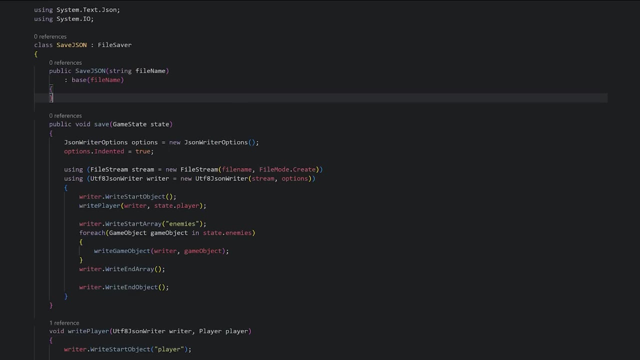 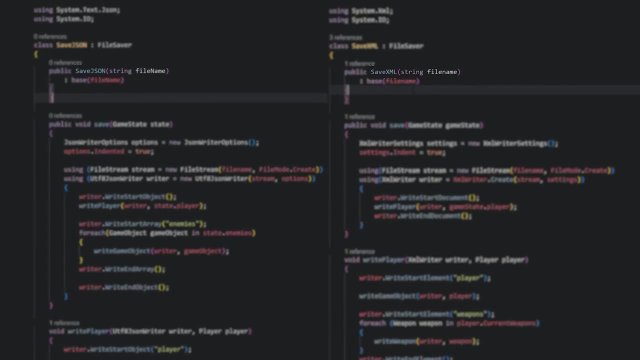 And our subclasses can grab it from this protected variable. But this is a bad idea. We've now coupled both of these classes to the same input. They must take a file input, So if there ever became a need to create something that didn't use a file, 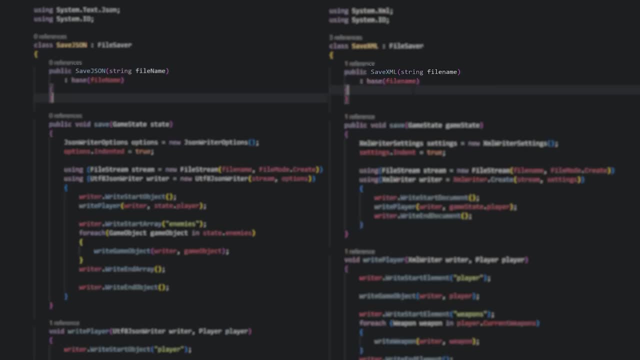 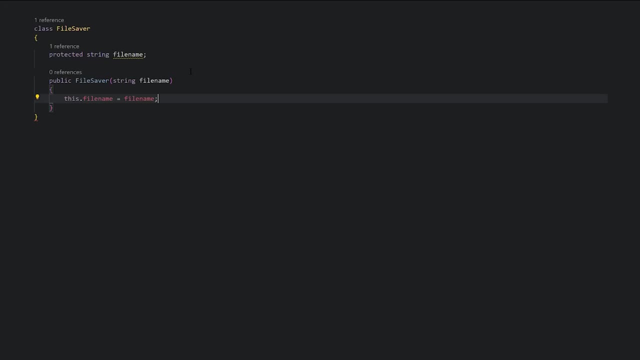 like a database or cloud connection. this would break the abstraction And, on the flip side, this abstraction brings us no value. What does this abstraction save us? Well, I guess we don't need to assign the variable twice, But this isn't any complicated logic. 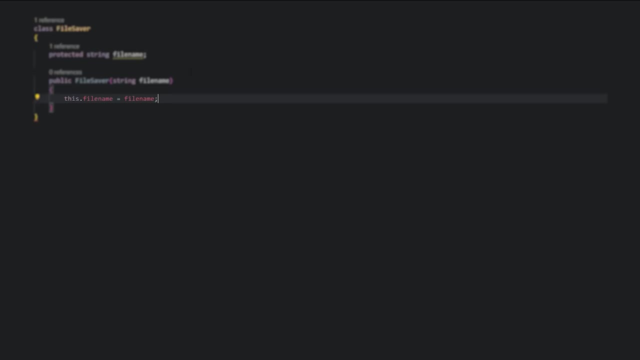 It's simply assigning a variable, So for me, this squarely fits into the not worth it camp. Okay, now what about the save functionality? We could consider creating an interface that represents the save method, But we do know that this would increase coupling. 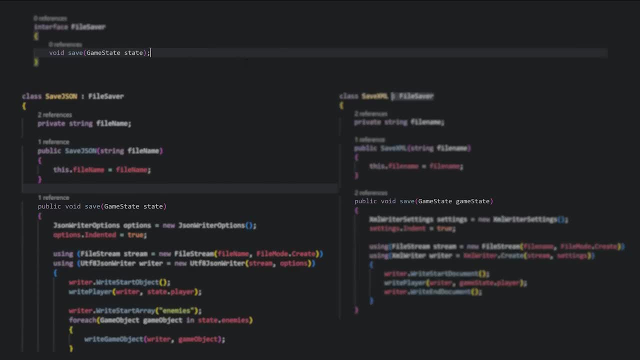 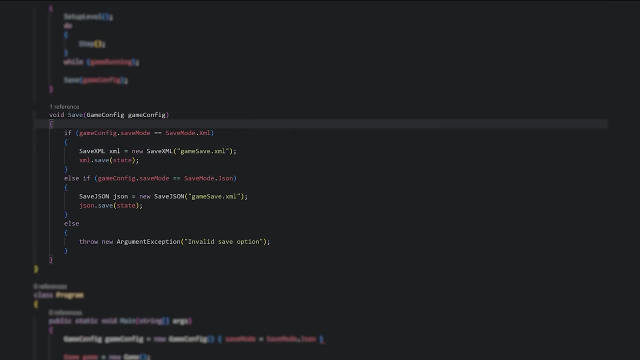 Because now both of these classes are constrained to the same save method. So what benefits does this abstraction bring us? Well, let's look at the usage. We have an if statement that decides which class to create and calls save on one of them. 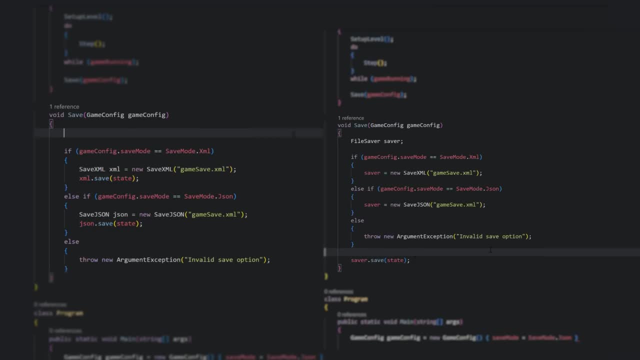 So if we add a common interface, we only get to remove this one duplicate save line. That doesn't simplify the program in any meaningful way, So I'd also put this into the. it's not worth it camp At this point. it's better to keep these as two distinct classes. 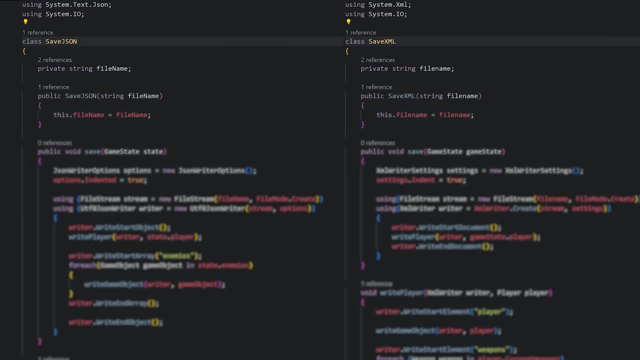 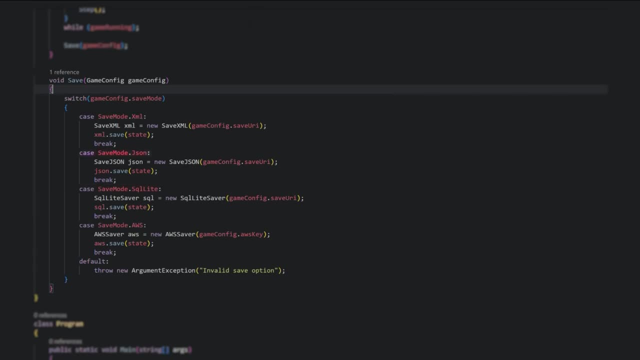 With no connection at all. There are two cases where it would make me decide it was worth it. One would be if we added more save options. If we had three or more, we might want to extract the construction of these save objects into a separate piece of code. 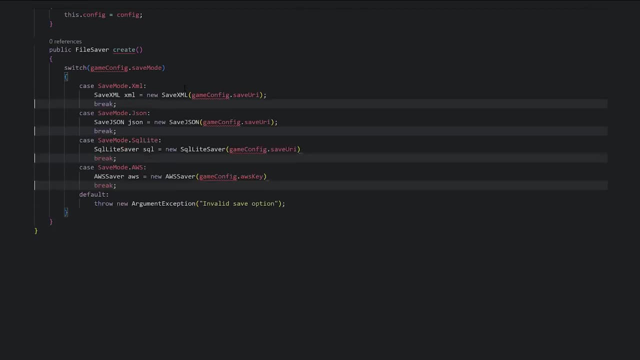 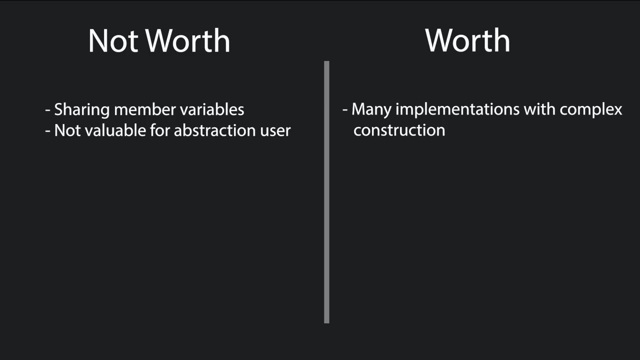 Especially if the different savers had different parameters, Like a database configuration. The other case would be if we needed our program to defer or repeat saving at a different point in the program, For example, if we wanted to save every five minutes automatically.